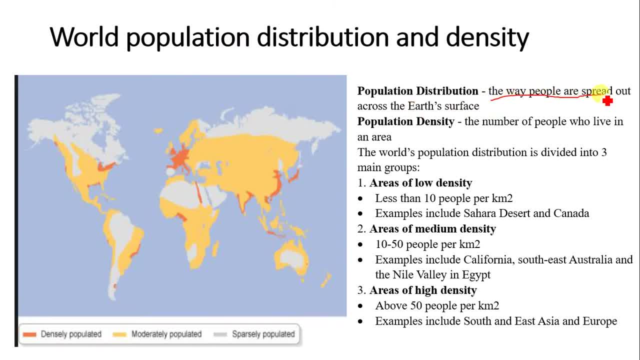 the word. population distribution is simply the way people are spread out across the earth's surface. the way people are spread out across the earth's surface And population density is the number of people will live in an area. So the number of people will live in an area. So you find out that the world population distribution is divided into three main groups. The world population distribution is divided into three main groups, So we have areas of low density. 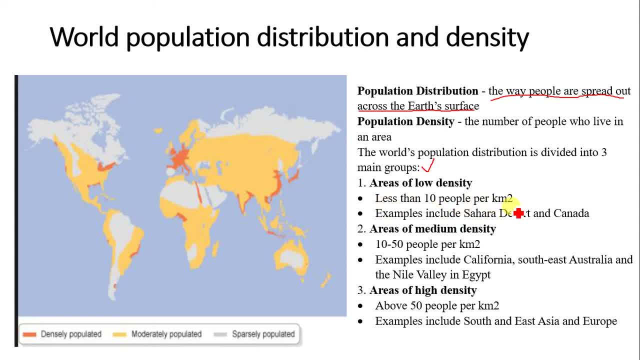 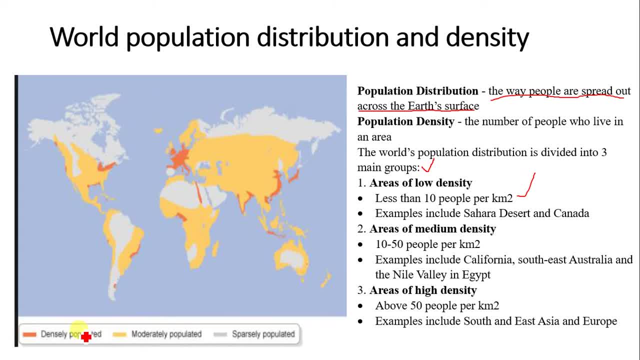 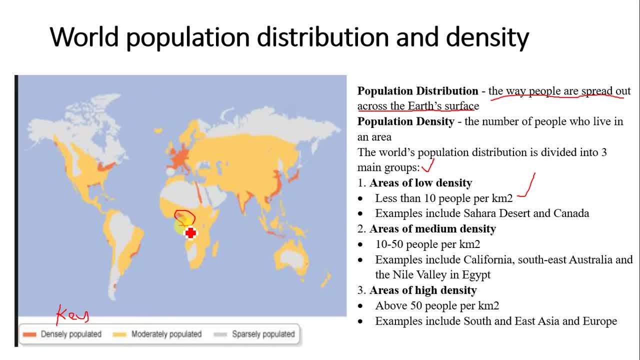 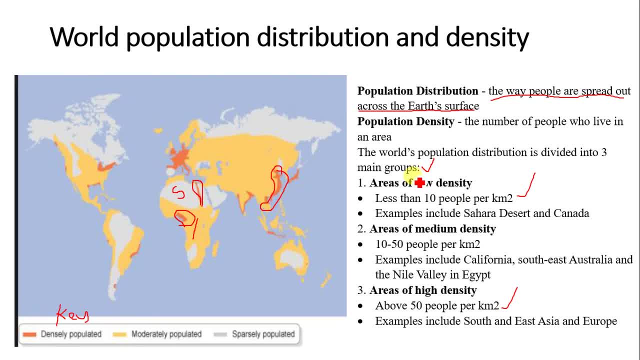 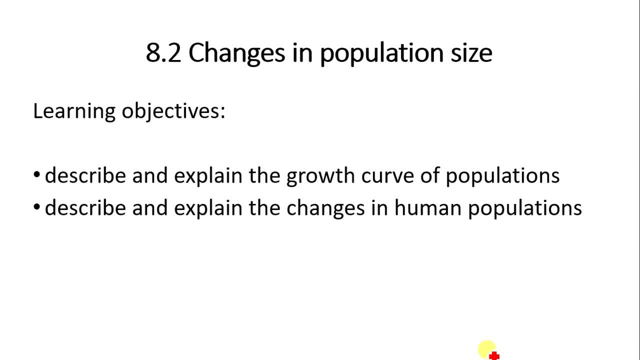 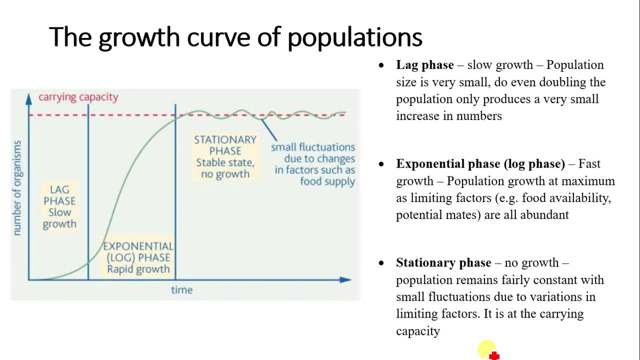 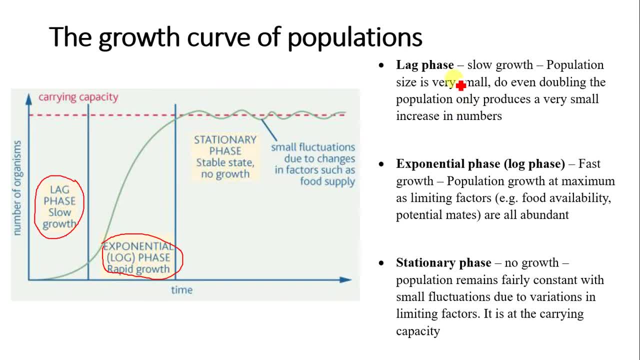 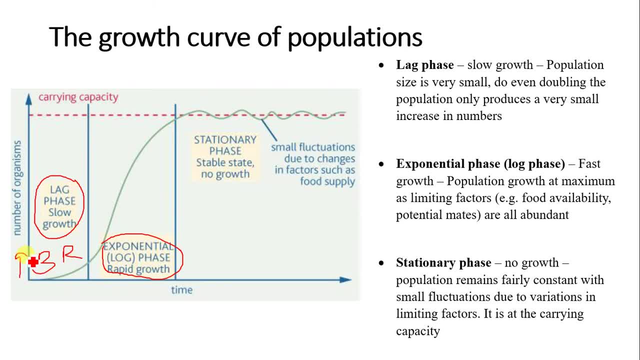 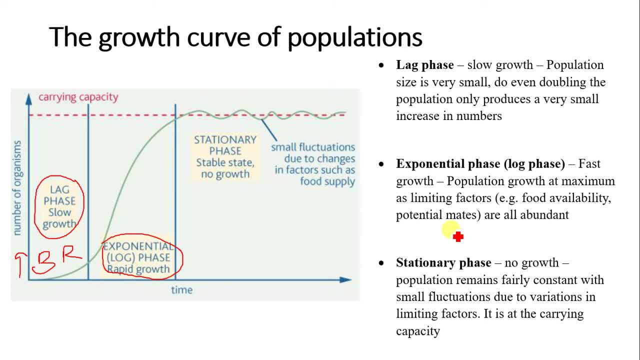 a criteria in this situation. so you find that the population growth is quite, very fast, food is available and there is availability of potential mate, so, as a result, the pet rate will be high and things like improvement in medical care is available. so you expect that the population, within this population growth, within this exponential phase, will actually 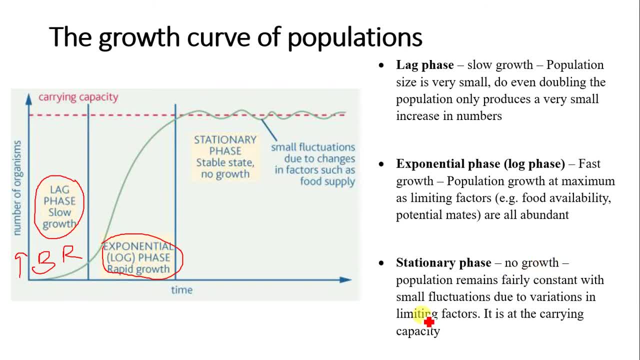 be very high. then we have stationary phase where there is no growth, population remain fairly constant, with small fluctuations. you see small fluctuations where it increases, decreases, increases, but it is usually around the world carrying capacity of that particular environment. now no growth, when population remain fairly constant, with small fluctuations due to variation in limiting. 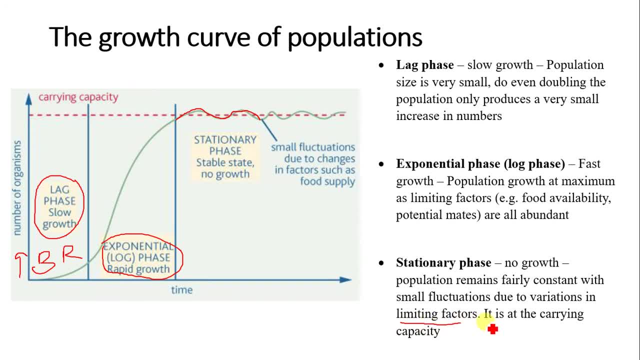 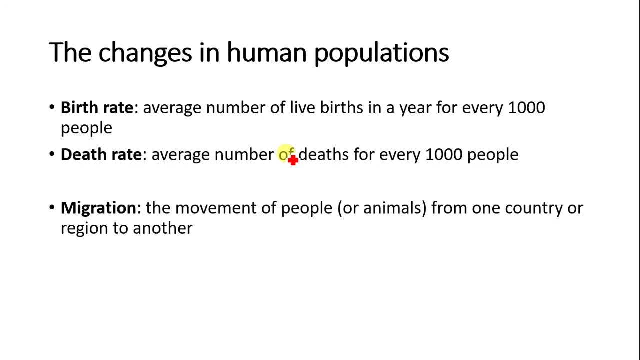 factors due to variation or the in limiting factors, that's, difference limiting factors. it is at the current capacity of that particular environment. so variation limiting factors, such as food supply, such as potential mate, this can actually lead to some fluctuations within the stationary phase. so now let's look at the changes in human population. changes in human population. 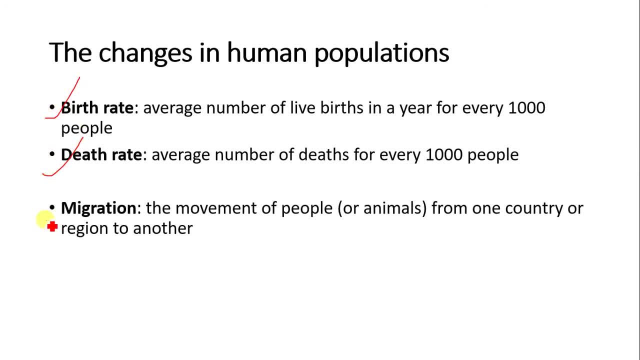 we have. look at bed rate, death rate and also population migration. so bed rate is the average number of life beds in a year for every 1 000 people. you can pause this and copy these definitions down. it comes out in between questions like a two mark, three mark questions at times. so bet is the average number of life bet in. 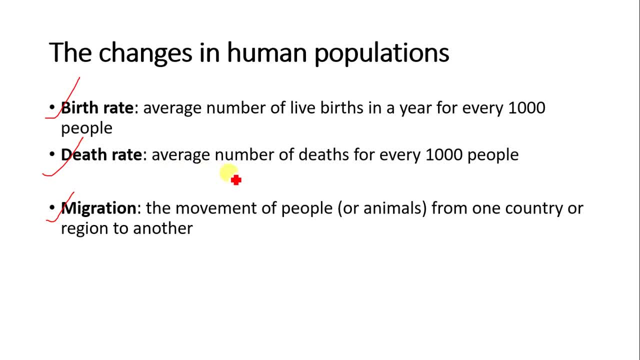 a year for every 1 000 people, while debt rate is the average number of debt for every 1 000 people, then migration is the movement of people or animals. you can see that in these last two examples the migration is integration. migration is the movement. 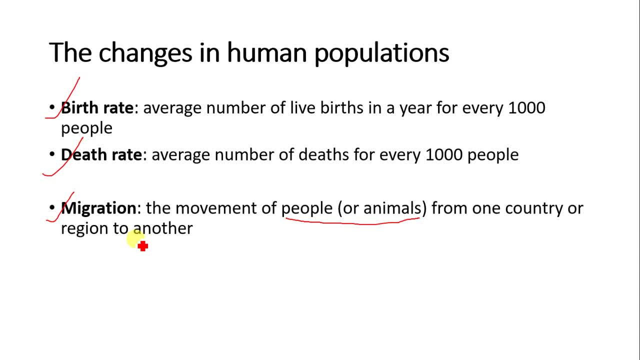 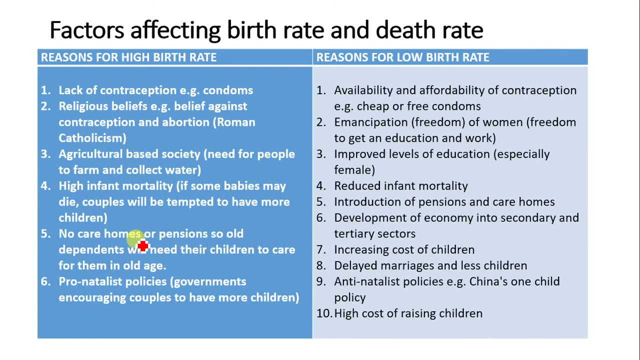 of people or animals from one country or region to another. migration is the movement of people or animals from one country or region to another. so we'll look at some of the factors that affect bed rate, death rate and also migration. so let's move reasons or factors affecting bed rate. 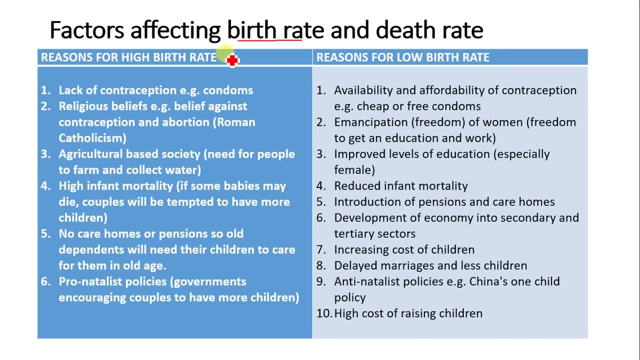 and debt rates. so what are the reasons for high bet rate and what are the reasons for low bet rate? so some areas, like that's less economically developed countries- less economically developed countries have less economical countries normally have high better it. why more economically developed countries usually have low better it. so 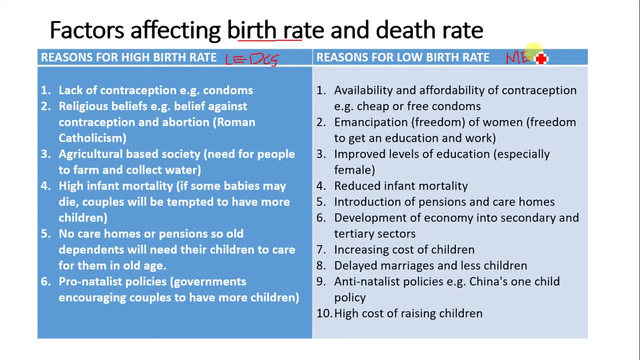 we now look at the reasons why some areas have high birth rate and some areas have low. better it so quickly. one reasons for high bed rate is lack of contraceptives. lack of contraceptives such as condom some. even if it is available, it is not affordable. that means it is quite expensive. 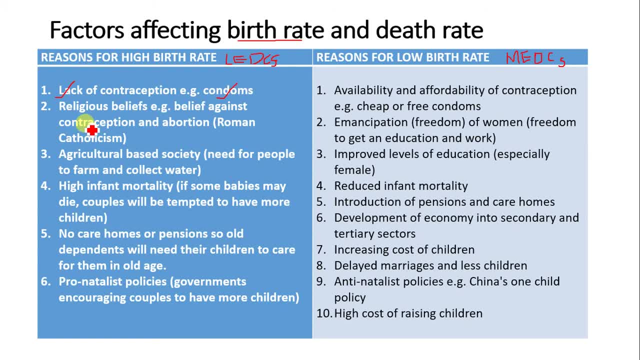 so people tend not to use it. so lack of contraceptives is an issue. then we have religious belief, religious belief such as um belief against the use of contraceptives and abortion and, majorly by roman catholic, don't believe in the use of contraceptives and they don't believe in. 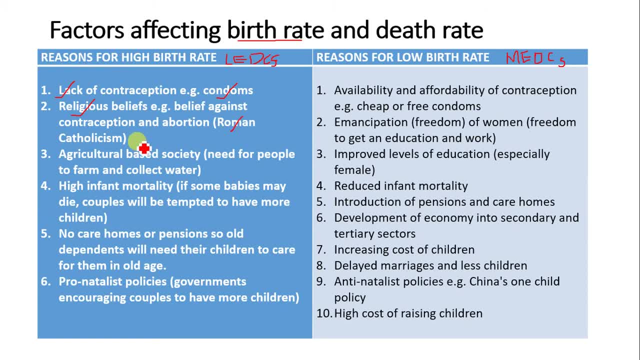 abortion. they only believe in natural method of bed control. um agricultural based society, like most lesser commonly developed countries, are into primary industries. so you find out that most of the people are into agriculture. so they need. they need the need for more people to farm and collect water, um in the case of irrigation, of irrigation process, so they tend to give better markets that. 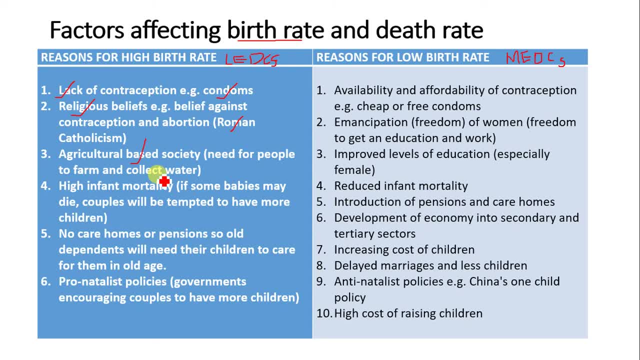 we assist them in the farming process. now, high infant mortality, that's if this, if some babies may die, uh, couples will be tempted to have more children, and this is as a result of poor medical care or poor medical availability in most of these less economically developed countries. 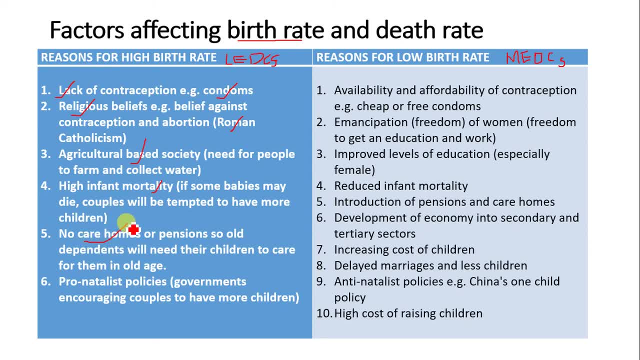 now no care homes or pension. so old people tend to be dependent on the on their children, on their kids, to take care of them during their old age. so they tend to give back to more kids. so if each of the kids send some reputants home then they'll be very good to it to be enough for. 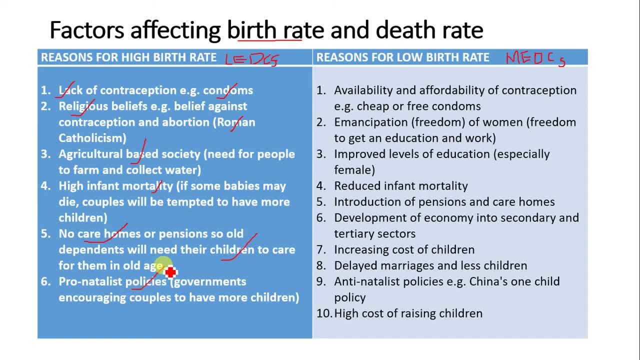 them to survive. then we also have pro-natalist policies, which are government encouraging couples to have more children. pro-natalist policies are policies where people are encouraged by the government to have more children. so if that is done, then you expect that the population will then- or the better, it will- tend to increase and population will rise in the same. 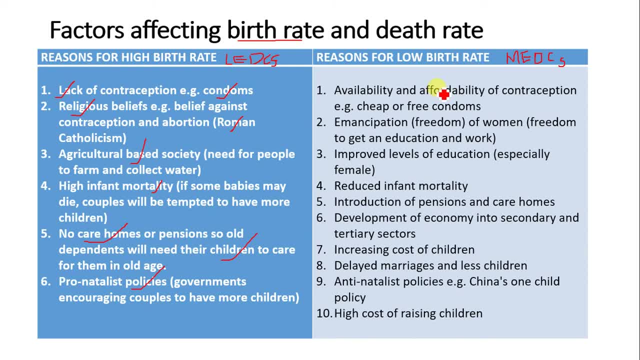 instance. then we now have reasons for low, better rate, such as availability and affordability of contraceptives in medc's. so if it is available and affordable- example, cheap or free condoms given to people- it tends to help reduce, better it. we have things like emancipation or freedom of 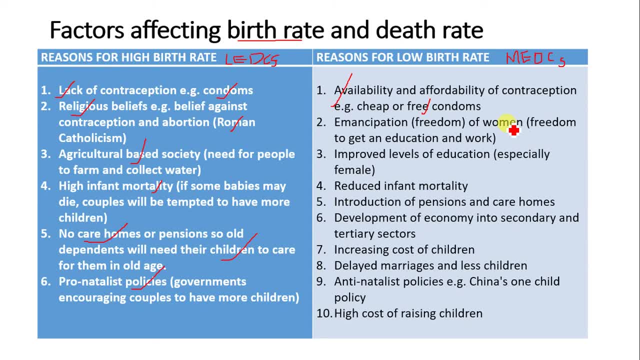 freedom of women to get education and work and this will help to increase their marital age and most women will now become career women so as a result, they might not have the time to give it to more kids. then we have improved level of education, especially women. now they tend to have 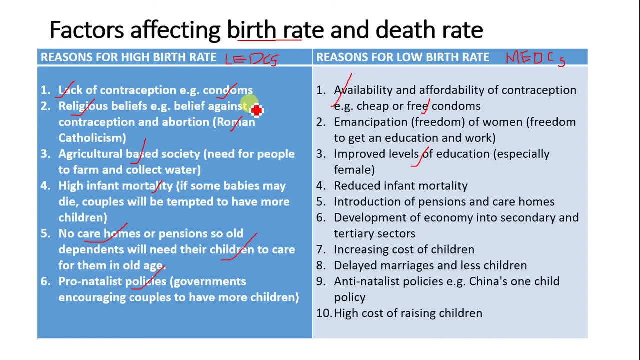 the ability to know the importance of contraceptives, to know the impact of high population growth. so if they are taught and they understand this concept, they tend to give that to to low number of kids and children. so low bed rate eventually reduce infant mortality, if you. 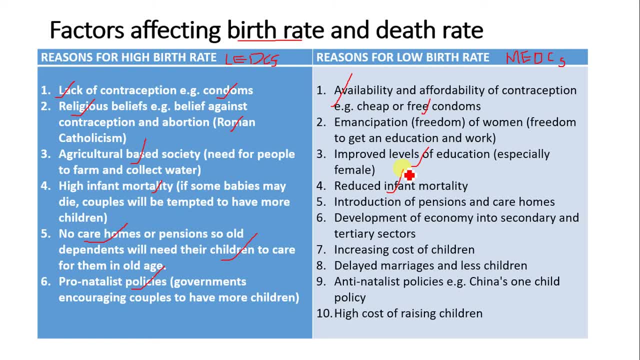 have an, if you have the belief that, um, the medical, uh the number of kids you give bed to, we tend to survive because you have good medical care and facilities within your country. you will not be tempted to give bed to a high number of kids with fear in your mind because some might. 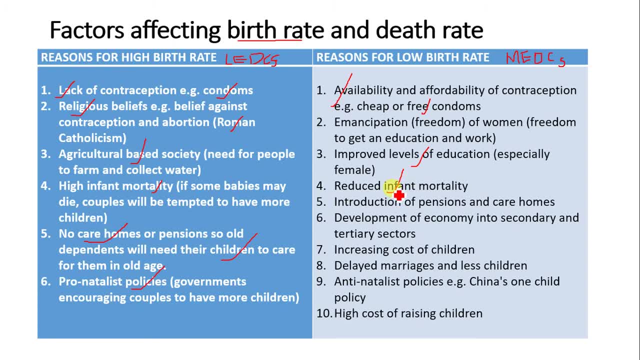 may die, but if you have reduced infant mortality, they tend to give bed to two, three kids and there's high possibility those kids will survive to a rightful old age. now, introduction of pension homes to care for the elderly so they don't depend on their children or on their kids at 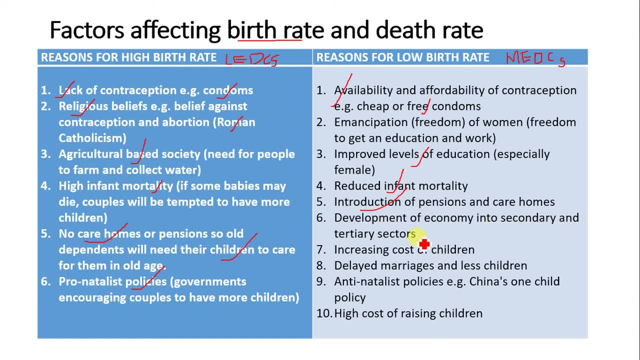 old age. development of economy into secondary and treasury sector. now in secondary and treasury sector you don't need more people, like in primary sector in agricultural based societies in less economically developed countries. so if the economy has transceded into a secondary or treasury sector, people tend to give back to low number of kids, so we have increased cost of. 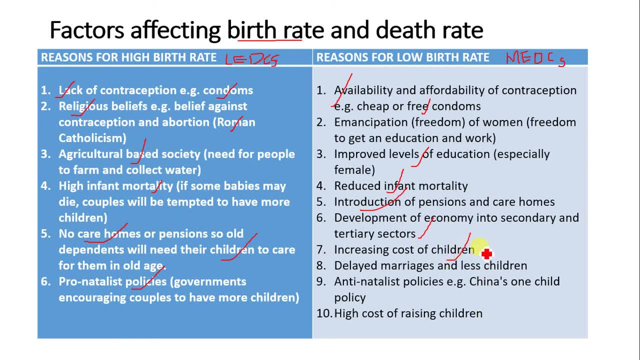 children. so there have been increased cost of raising children in the last decade, so people tend to give back to less number of kids which their financial capability will be enough to raise. then we have delayed marriages and less children. delayed marriages and less children in medc's. then we have anti-natalist policies like that of china, where people are discouraged from. 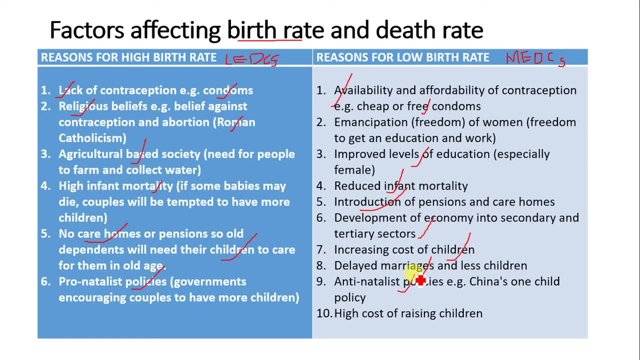 giving bets to. from giving, uh, from giving bets. so as a result, it drops the general population and we have high cost of raising children. also, i think this is tied to this. so please take note of all the these important point. at least you should be able to constantly list five out of the individual truth. 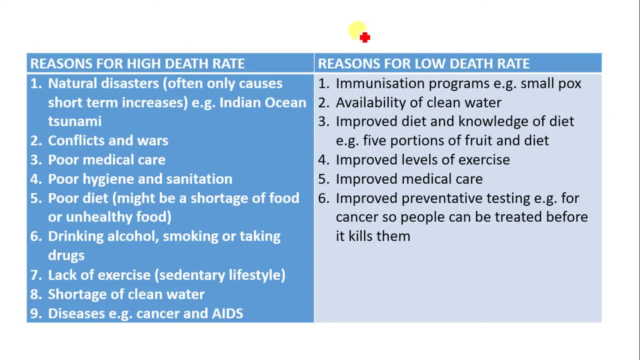 so we now have- we've looked at better it. so let's look at debt rate. so reasons for high debt rate: so there is high debt rate through in most ledc's and in medc's the debt rate is quite low. so let's just look at that quickly. so reasons for high debt rate: we have natural disasters. 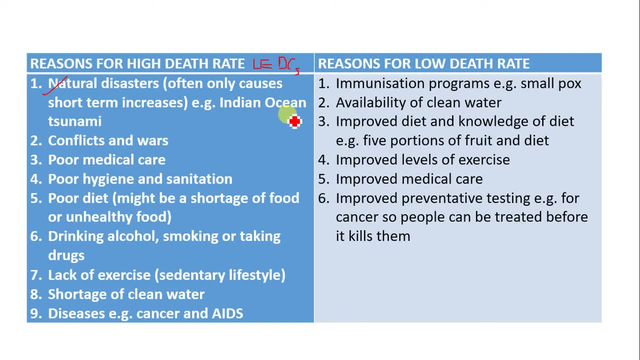 which often only causes short-term increase, like indian ocean tsunami. we have conflict and wars which lead to high death rates. poor medical care, poor hygiene and sanitation will need to increase in diseases and therefore affects the better it deteriorates. sorry, we have poor diet, might be a shortage of food or unhealthy food. you can't also lead to. 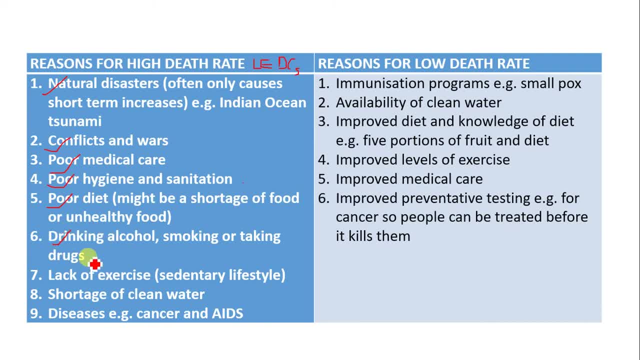 rate. drinking alcohol, smoking and taking drugs can lead to death rate. lack of exercise, where you have a sedentary lifestyle, where you just your life is simply based on a single location- you just sit, always without exercising your body, it tends to lead to high death rates. 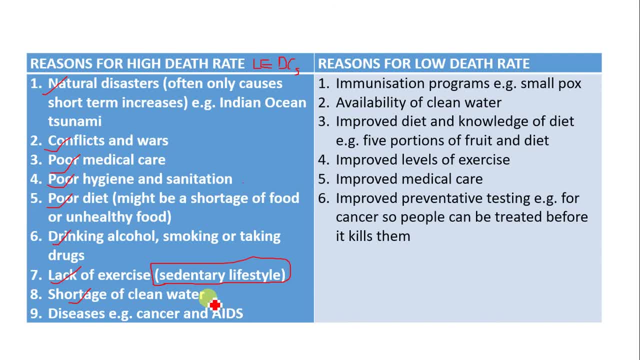 then we have shortage of clean water can lead to waterborne diseases and and disease also such as cancer, hiv and aids, and presently covid all has increased uh death rate. but uh, there are certain reasons why the world population death rate has also dropped, and some of these reasons include: 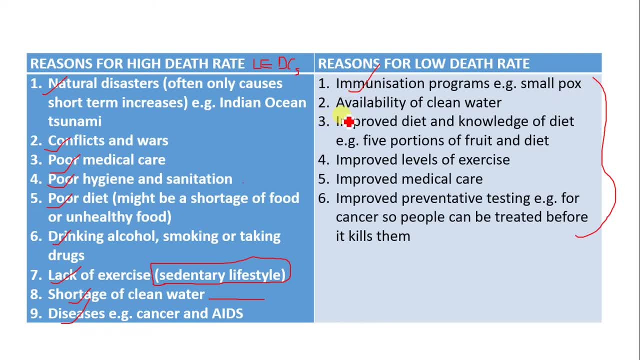 immunization program against smallpox. we also have an immunization program against covid going on presently, where people have been vaccinated. now we have availability of clean water. improved diet and knowledge of diet has also helped to lower the death rate. improved level of exercise. improved medical care, improved preventive testing. 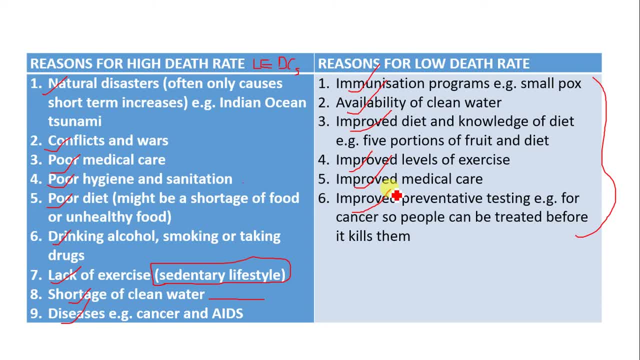 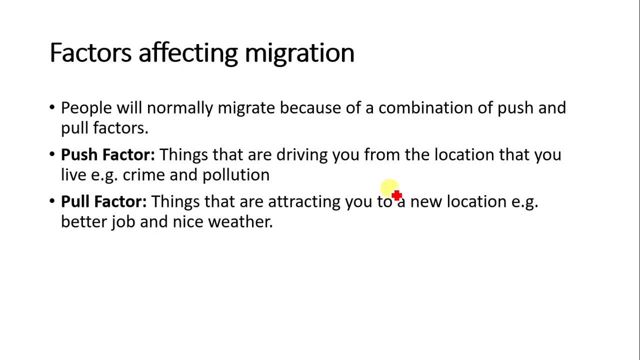 example, are for cancer, so people can be treated before it kills them. so all these are some of the factors that have led to low death rate. so factors affecting migration. now, people will normally migrate because of a combination of push and pull factors. so what are the push and pull factors? so push factors, these are things that are: 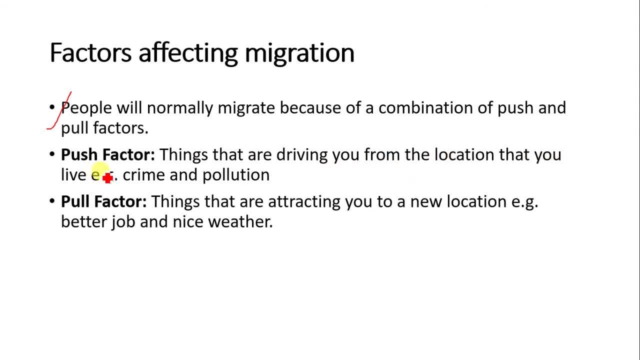 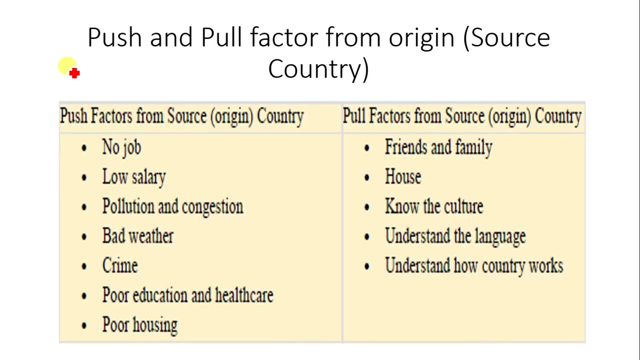 driving you from the location that you leave, things that drives people away from the location that they leave. examples are crime and pollution. these are push factors. then pull factors are things that are attracting you to a new location, and examples are better job and nice weather. these are pull factors to a particular location. then what are the push and pull factors? from origin? 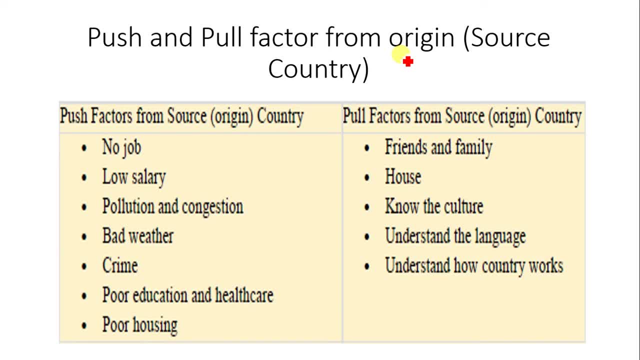 so what are the push and pull factors from our origins, source country? so push factors from source, that's, origin and things that drive people away from their country. uh, when there is no job and low salary, pollution and congestion. when you have a bad weather, there is high crime rate, poor education. 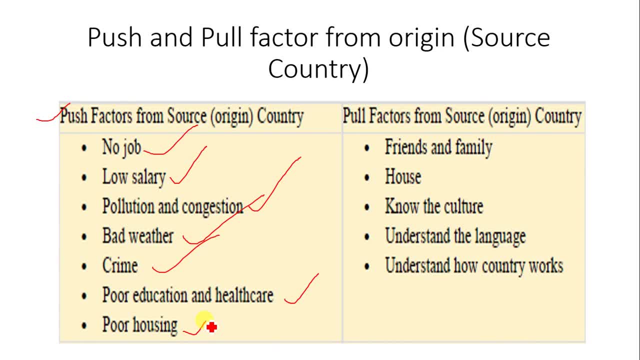 and health care and poor housing can actually be a push factors. and what are the pull factor from source or origin a country? so you see, what are the pull factors from source or origin a country. so you see, um, we have family and friends, we have house, we have, you know the culture, you understand the. 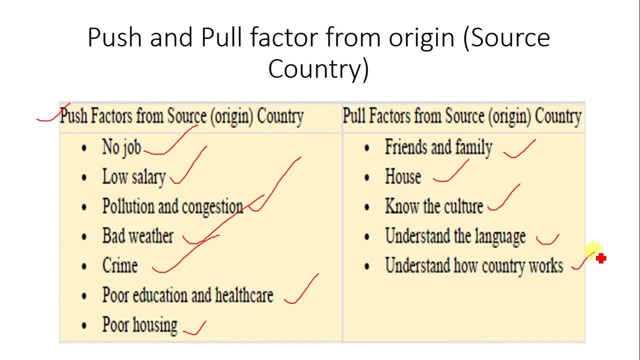 language and you understand how the country works. so these are the reasons why people will tend to remain in their country if all these other factors are present. so these are the pull factors to the source from source. that's the origin of that one country. so if you leave your country for a better 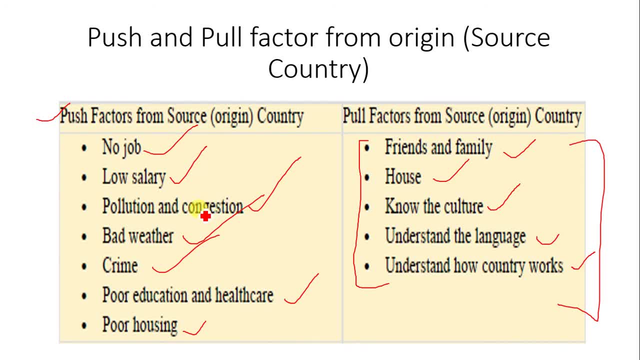 job, for high salary, for a sanitation and good weather. so the only thing that will make you remember or you want to go back to your country is majorly because of our friends and family. you know the culture, you understand the language, you understand how the country works. so let's. 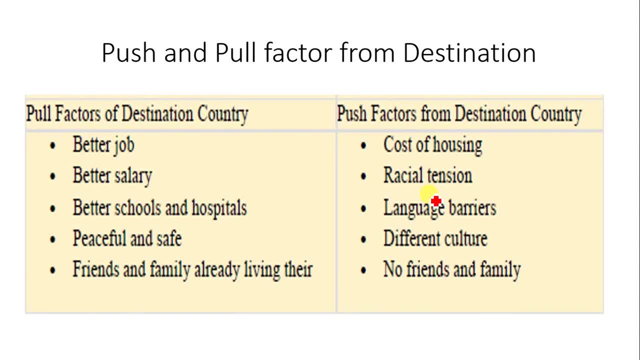 look at um push and pull factors of destination country. so what are those things that we attract you to the country you uh intend to go through? some of those things are better job, better salary. where you have a better school and hospitals, it's usually a peaceful and safe. 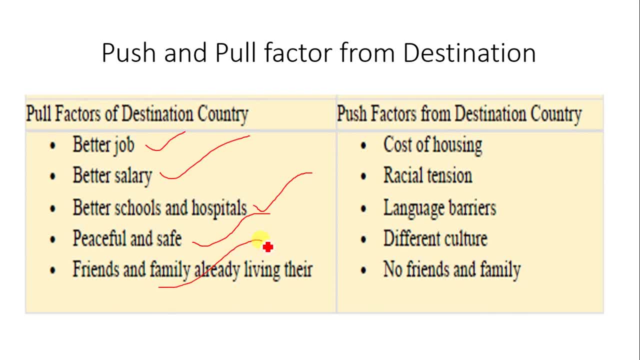 environment, friends and family are already living there, so it will be easy for you to move over there. but in a situation where- what are those things? that, and once you go to the country, that might be an issue that will make you leave that particular country, back to you, to your original, 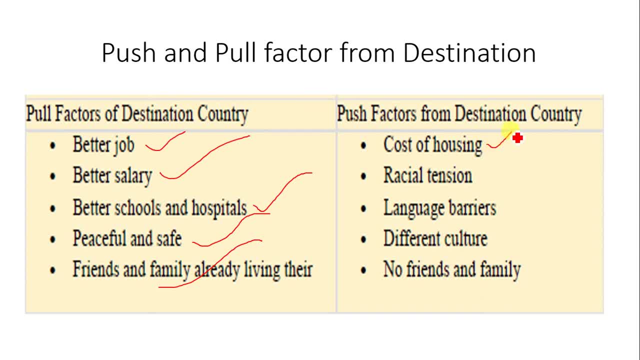 source is maybe when you travel. you now have issues with cost of housing quite expensive. you have racial tension- they abuse you racially- and language barriers. you don't understand the language. if you have an english-speaking country and decide to go to a francophone country, it's a very big issue. if you don't know how to speak french, then we have different culture. 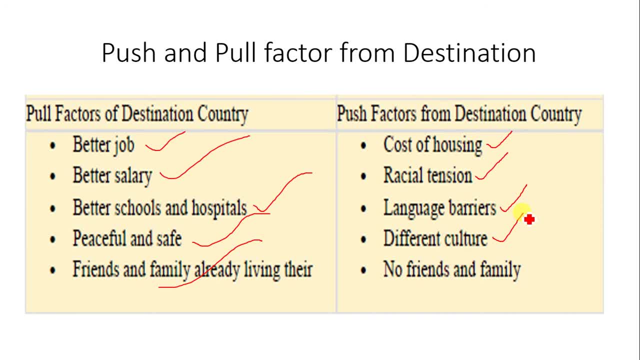 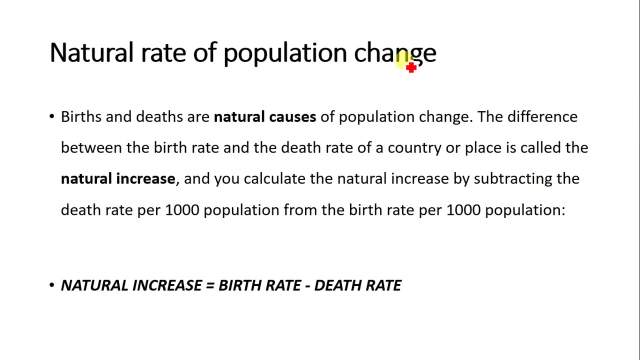 possibly you don't understand the culture and if you have no friends and families there, you tend to be very bored and at times you might be a reason for you to return back to your original country. okay, so natural rates of population growth or population change you see in the exam. they normally ask: 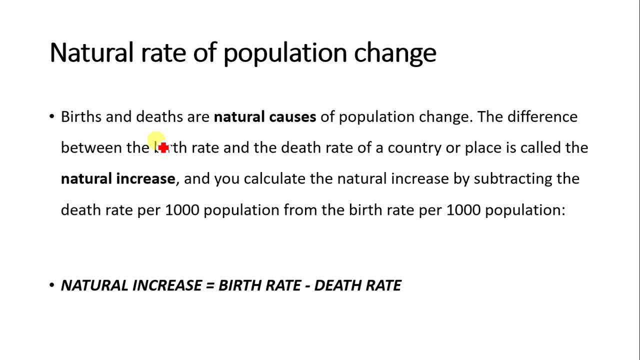 questions on this, where you just have to calculate the natural rate of population change. so you see birth and death rate and death and natural causes of population change. so the difference between the bed rate and death rate of a country or place is called natural increase and you calculate the natural increase by subtracting the debt rate by one thousand. 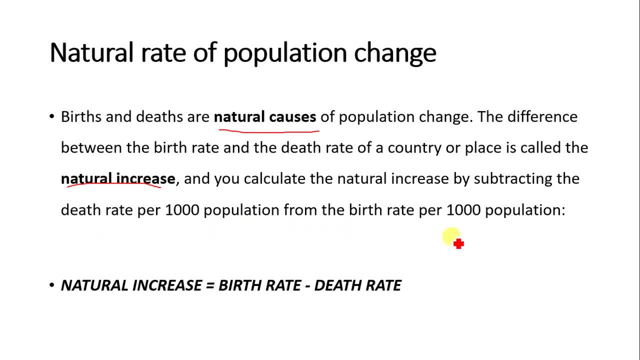 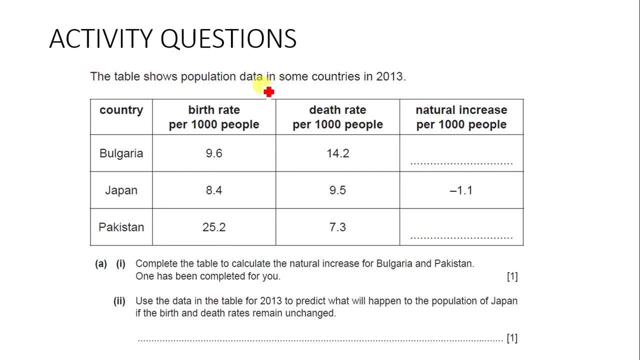 population from the birth rate and per 1,000 population. So natural increase is birth rate minus death rate. So simple: Once you get the data, you just subtract, you get the answer. So I have a sample exam question here where they said the table shows the population data. in some 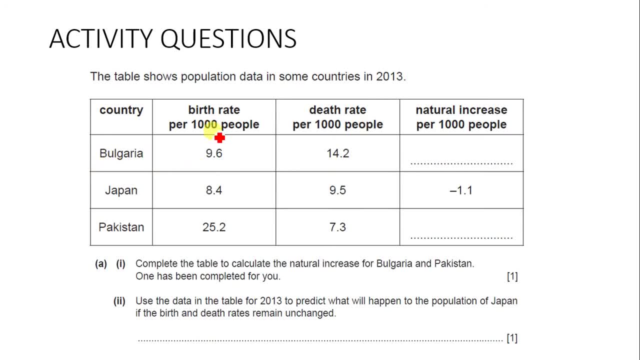 countries in 2018.. We have Bulgaria. we give us birth rate and death rate, the natural population increase. The first question is: complete the table to calculate the natural increase for Bulgaria and Pakistan. Natural increase, remember, is birth rate minus death rate. So in this case, 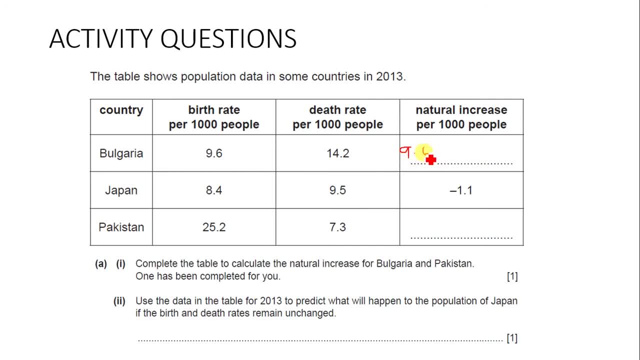 it will be 9.6,, 9.6 minus 14,, 14.2,, which will be equal to. then this will be 25 minus 7.3,, which will be equal to. so let's just look at the answers quickly. 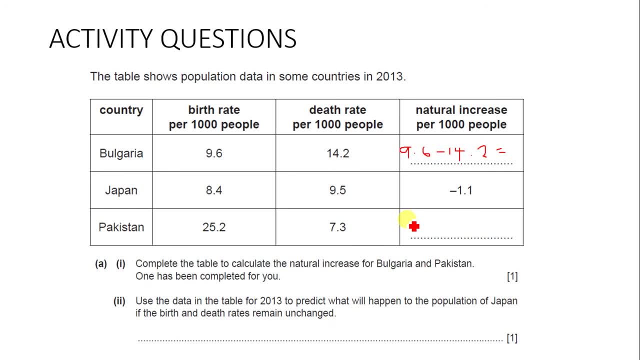 So here will be 25.2 minus 7.3.. So let's clear: 25, 25.2 minus 7.3, 7.3.. This is 17,, 17.9.. Oh, sorry, 17.9.. 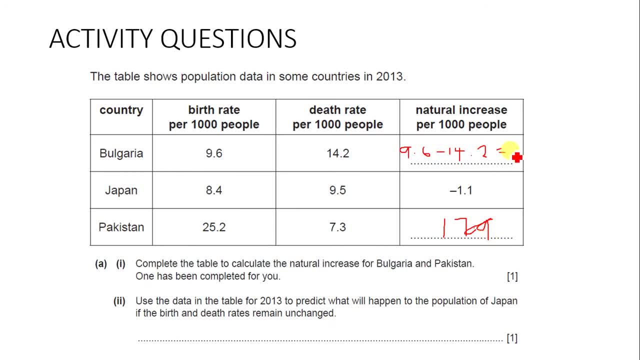 Why this? We give us 9.6 minus 14.2.. This is minus minus 4.6.. That means the population is decreasing. There is no increase. Naturally, if there's a growth, it might be due to migration. 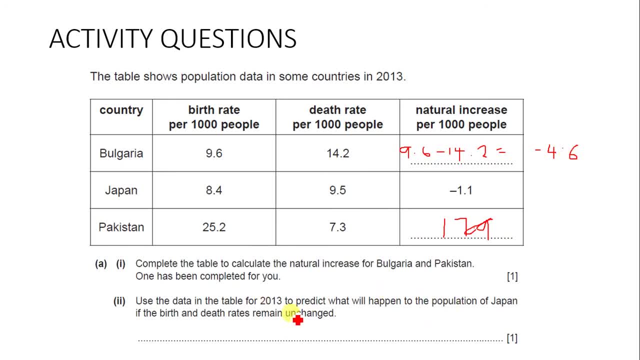 14.6.. Now we are done. That's one mark, They say. use the data in the table for 2013 to predict what will happen to the population of Japan if the birth and death rates remain unchanged. Japan population will decrease because it's at minus 1.1.. So simple, Just come right: decrease. 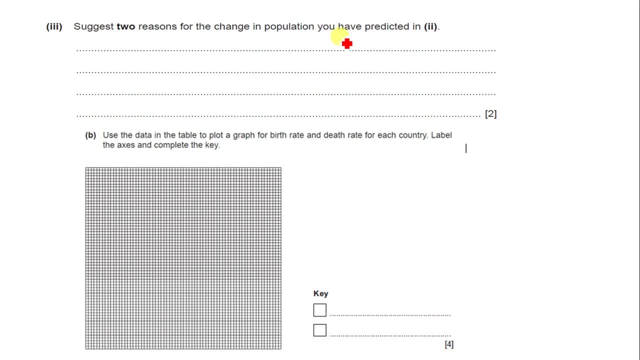 So this suggests two reasons for the change in population you have predicted. So the two reasons for change of population you have predicted in Japan. So improving medical care. So what are the reasons for low birth rate? That's what they are asking you, because the birth rate is quite low. 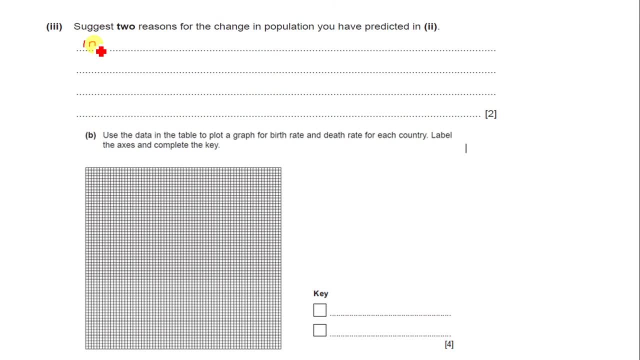 That is why you find that the population, natural population growth rate is less. So improve medical care, That is, it reduces infant mortality. That's one. You can look at availability of contraceptives: That's two. Most of the economy is within a secondary and tertiary sector of the economy. 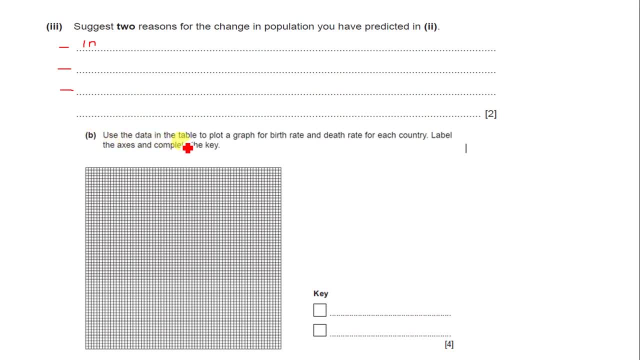 I mean, that's three. So simple that you now have used the data in the table to plot a graph of birth and death rates for each country and you label your assets, So you should be able to use your key- label your assets- to draw this data for each country. 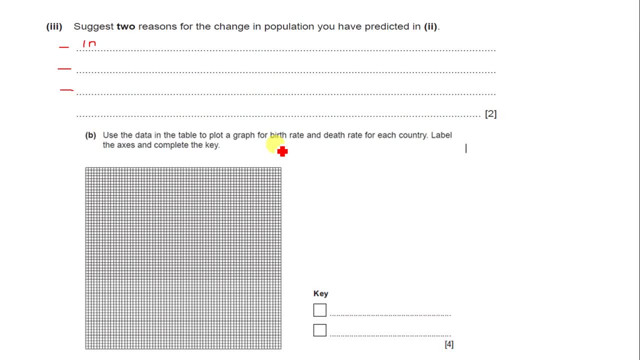 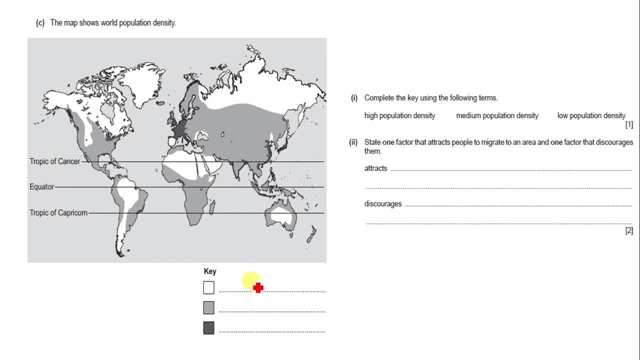 There is usually- it's usually a bar graph. So is this this? this is quite straightforward that you see, a question about population density I was talking about earlier. You see, they give you the key as a complete, the key using the following terms: high density population, medium density and low density.